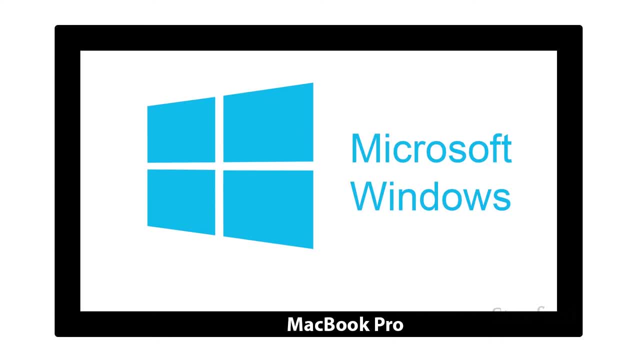 So suppose I start working in a lab and it turns out that that lab requires me to use some software and I can't run it on my Macintosh because it doesn't run on Mac OS. I can actually replace Mac OS with Microsoft Windows on my Macbook Pro hardware. 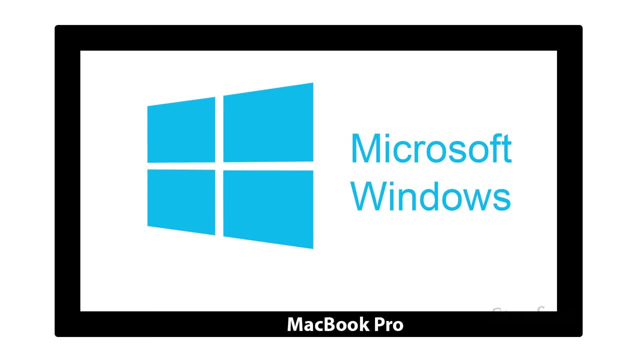 And that's because- Because the operating system is actually software as well. So those are the instructions that we think of as being an integral part of the computer, And they're actually not. They're just instructions running on the hardware. Similarly, if I decided I wanted to take my laptop here, 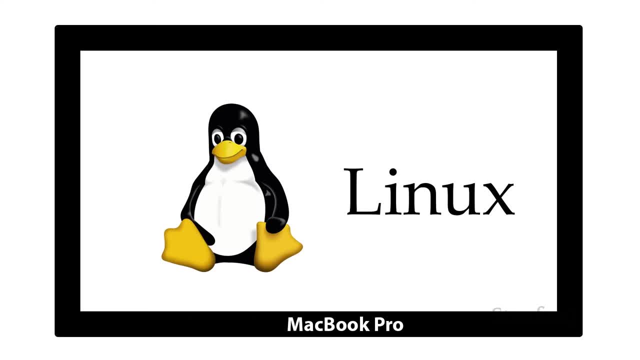 and turn it into some sort of a server and I wanted to get Linux software for it. I can go ahead and replace Mac OS with Linux And again, that's because the system software is replaceable and that is something, a set of instructions. 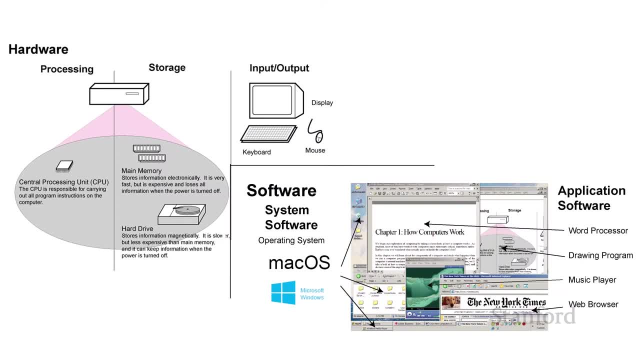 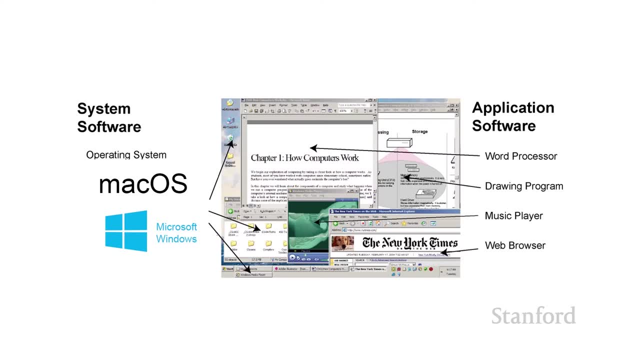 that runs on top of the hardware. So we have this distinction between software and hardware, And we have a distinction between application software and system software, And we're going to take a closer look at the system software and the operating system in another lecture. 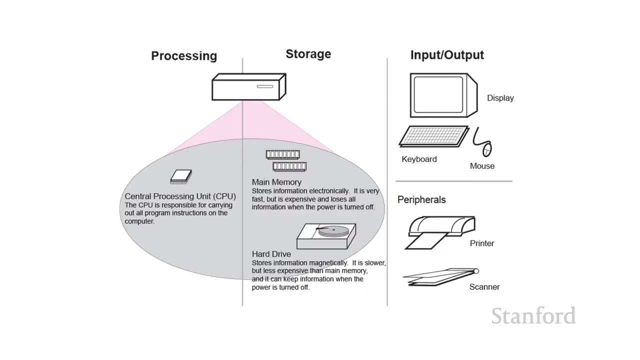 All right, let's focus on the hardware itself. We distinguish between three main categories of hardware. We have processing, which is primarily the central processing unit, and then we have memory, which consists of two types of memory. There's primary memory and secondary memory. 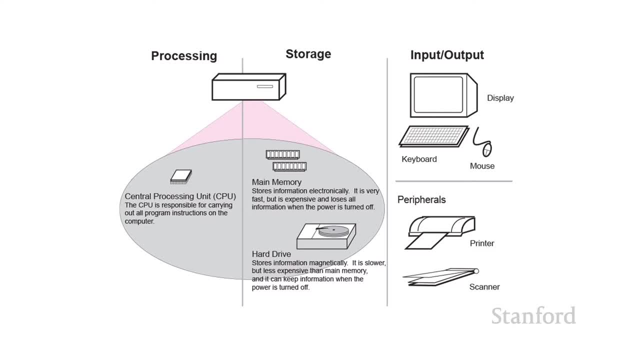 where primary memory is colloquially thought of as RAM, although it turns out there's a little bit more to it than just the RAM- And the secondary memory are things like the solid state drive, the hard drive, flash memory And basically the distinction between the primary memory. 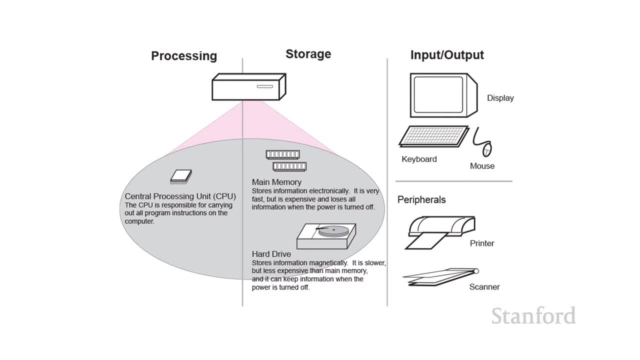 and the secondary memory is. the primary memory is what we refer to as volatile, So if the power goes out, I lose all the information in the primary memory. The secondary memory is non-volatile, which means even if I completely lose power, the information in secondary memory is still fine. 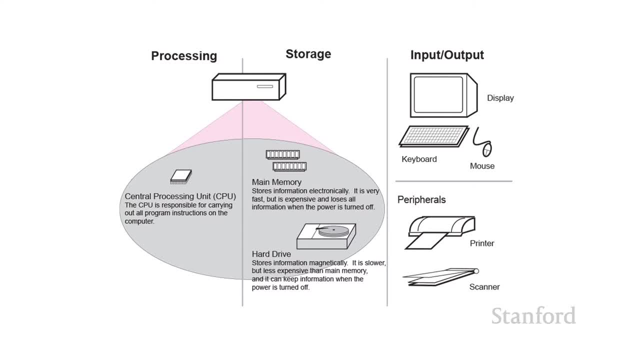 The other main distinction is primary memory is much, much faster than secondary memory. because you may wonder why don't we just use this non-volatile memory? Well, the answer is because it's much slower. Now, I also should highlight here: 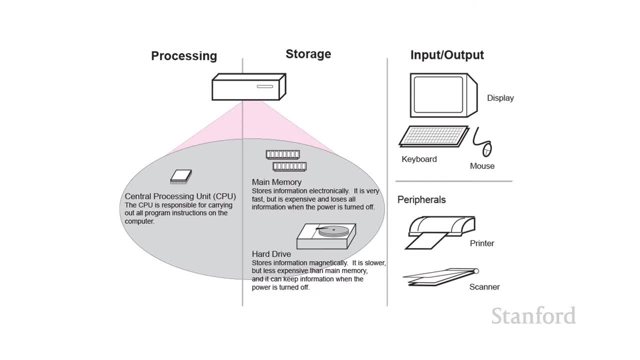 that nowadays, this distinction between primary and secondary memory or, more pointedly, volatile versus non-volatile memory, It's a little bit hidden because we're used to being able to put our laptops or cell phones or tablets to sleep and turn them on later. 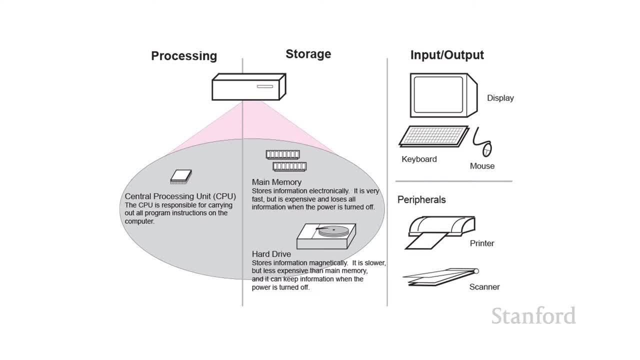 and everything's still there exactly as it was before, And it turns out that when we put a computer to sleep, the main memory is still getting a little bit of trickle charge of electricity. If the battery goes out completely, you're going to lose all the information. 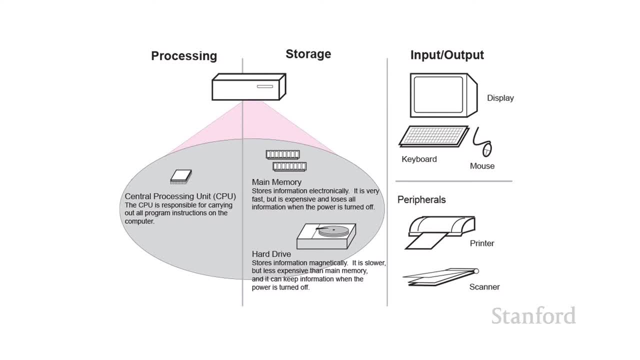 So, in addition to processing and memory, there's also input output, And that includes things like the obvious, the display, the keyboard, the mouse, if you've got one, And it also includes external devices like printers and scanners. I should also mention that, while I'm primarily 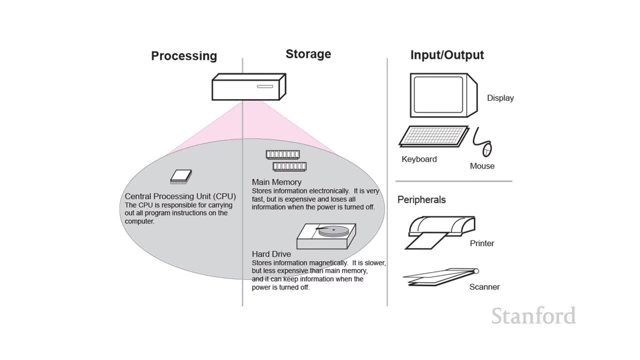 going to be focusing here on laptops and desktops. smartphones and tablets work almost exactly the same. They have the exact same distinction between primary memory and secondary memory. They've got that processor with a central processing unit, And modern smartphones and tablets also have a graphics processing unit. 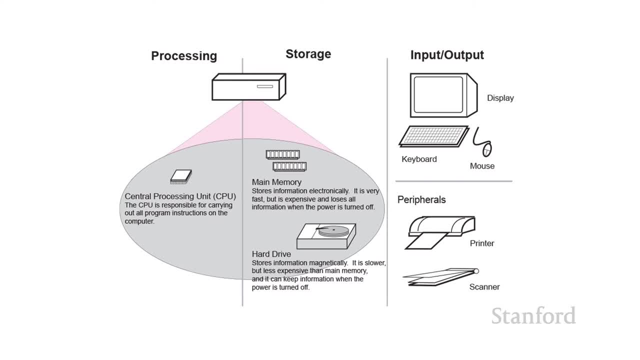 And then, finally, there's something in terms of input output. I suppose, in some sense, that the display is acting as both an output and an input for smartphones and tablets, But in addition to these types of computers, there's also what are referred to as embedded computers. 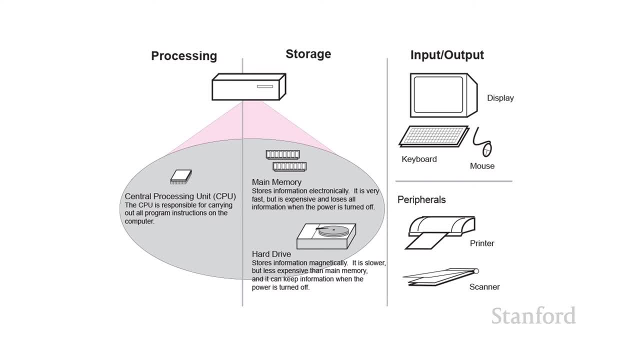 or embedded systems, And embedded computers are the computers that run inside of things like our car. So our car has computers that are tracking different pieces of input, Like how hot is the engine, How much fuel do I have, How hard is the user pressing on the gas pedal? 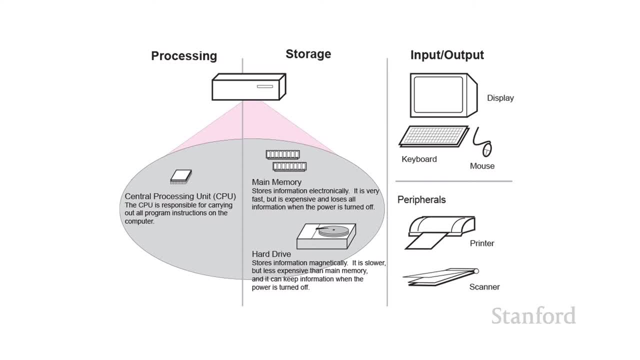 These are the sorts of inputs that come into the embedded computer that's inside of your car, And the outputs would be things like: how much flow of gasoline should I let into the engine? So there's lots and lots of different computers other than just the desktops, the laptops, the smartphones. 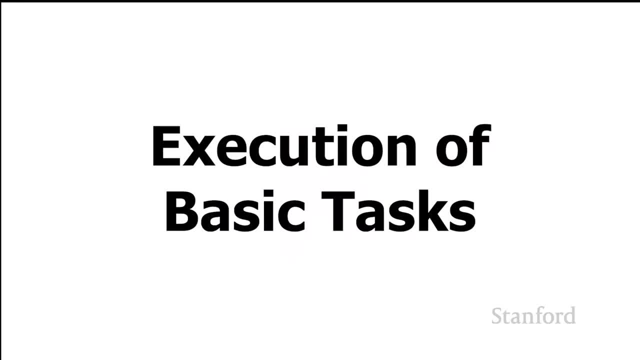 and our tablets. OK, So what I'm going to do now is we've gone over processing with a central processing unit and a graphics processing unit, We've gone over our memory with the primary and secondary memory, And what I want to do now is see how these different components 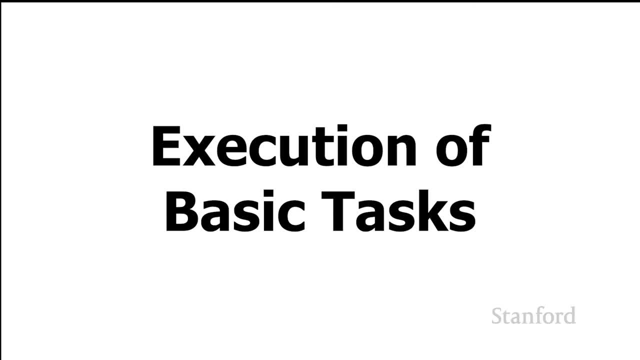 kind of play out when I'm carrying out some basic computing tasks. So let's start off with I'm going to install an application, So I mentioned before: hey, I need to get a hold of Premiere Pro. So what is that all going to involve? 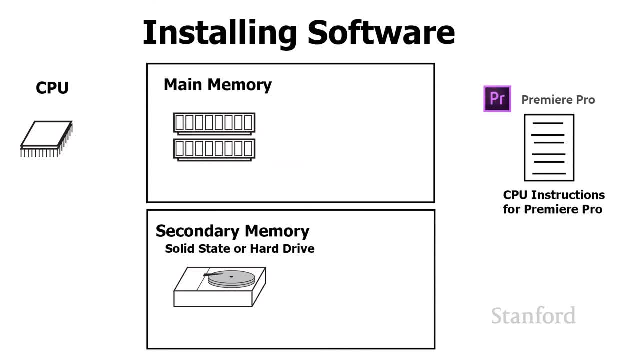 Well, Premiere Pro consists of a bunch of different instructions, And so I need to get a hold of those instructions and get them onto my computer. So I'm going to go ahead, I'm going to download a copy of those instructions And I'm going to install on my computer. 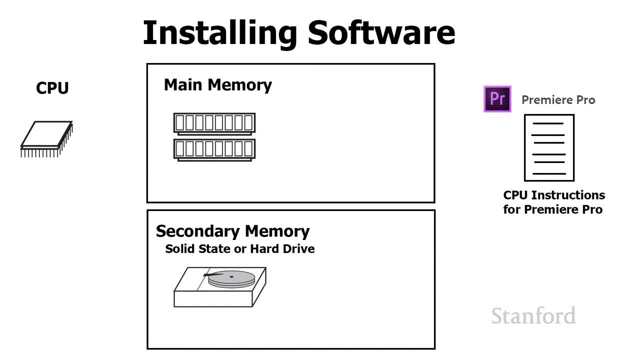 Now it turns out a lot of times when I'm installing these programs, the programs that I'm actually getting over the internet, or sometimes when I'm buying a CD-ROM or DVD copy of a program, it's actually those programs are actually compressed. 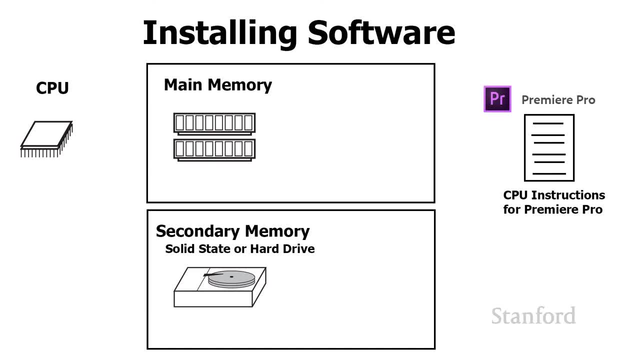 So we talked about compression last week, particularly if you're installing over the internet. But again, also sometimes when you're installing from a DVD or CD, the files are compressed in order to allow it to transfer through the internet, taking less space, which makes things cheaper for whoever's. 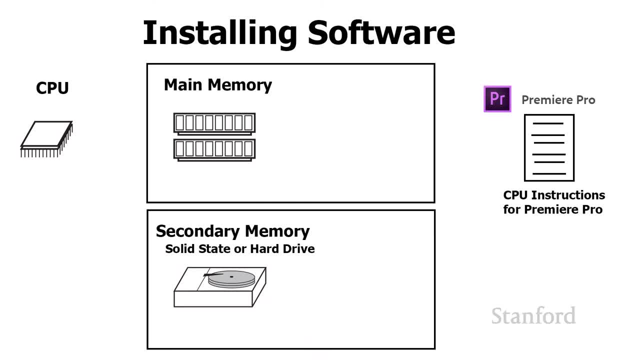 paying to serve up those files. So when they come over to your computer, they do need to be decompressed. Sometimes there's a two-step process that actually decompresses all the files onto your hard drive And then, after they've been decrypted. 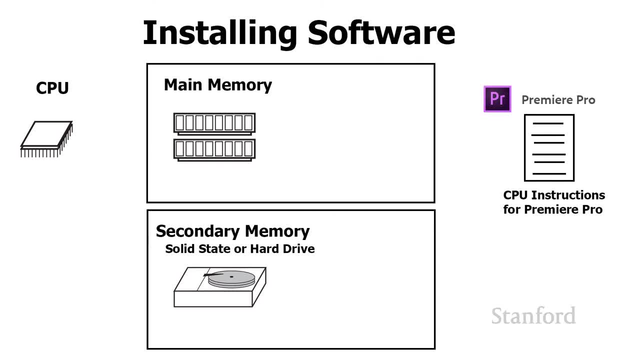 you have to run an additional installation program. So that's what's going on with that. So I need to get the files, I need to get the installation files onto my computer And I need to decompress them and get the instructions onto my computer. 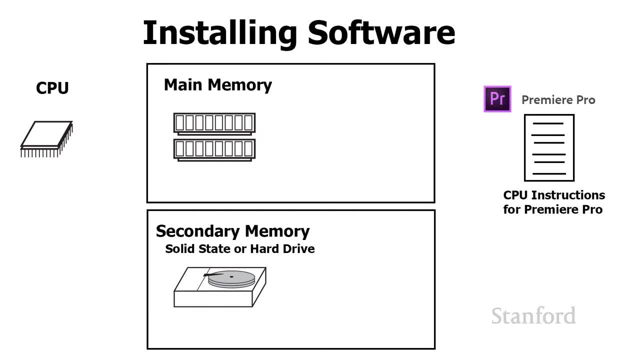 Those instructions, since they're things that I want to have stick around even when the power on my computer goes off. therefore, those instructions need to go on my secondary memory device, whether it's a solid state drive or a hard disk. Ultimately, the instructions after I'm done installing. 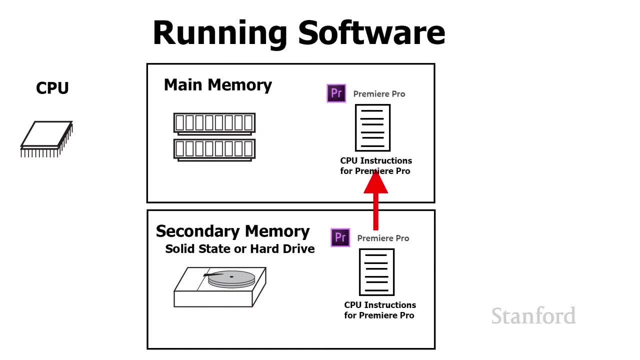 are going to be on that secondary memory device. Now, when I run an application, what happens is the instructions need to be copied into main memory, because it turns out the central processing unit cannot access things directly on the hard disk or the solid state drive. 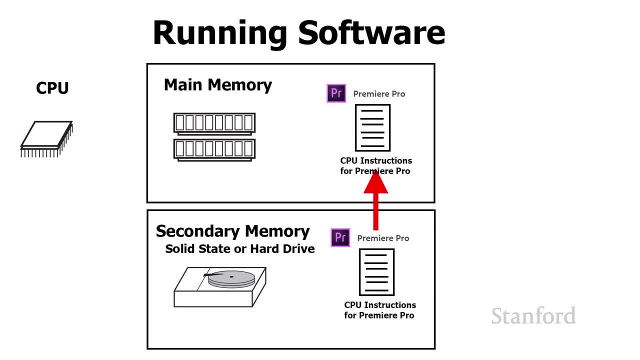 So if my program is actually going to execute, as opposed to the program is just installed on my computer and I'm not actually running it. if it's installed on my computer and I'm not actually running it, then the instructions are on the hard disk or the SSD. 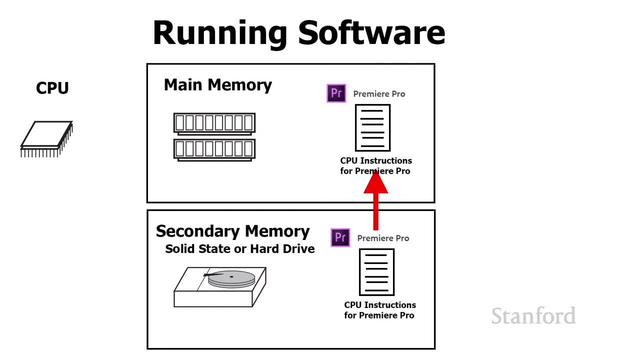 When I actually double click on that, it's going to be on the hard disk. Or I tap on it on my cell phone and it starts up. The instructions are going to get copied from the solid state drive or the hard disk. They're going to get copied into main memory. 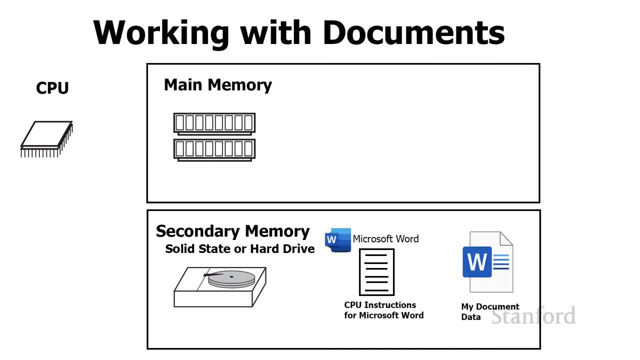 where they can actually get access by the CPU. Now, as far as documents go like, let's say, I'm, I decided I want to open up a Microsoft Word document, Those documents- when I'm not accessing them directly from a program, they're going to also sit. 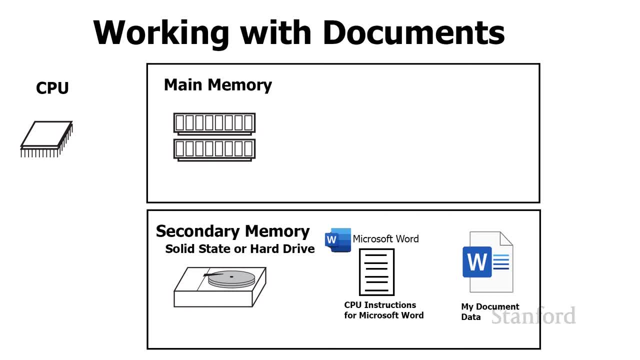 in that secondary memory device because I want to keep my internet. I want to keep my production humanities paper. I want to keep that around after the computer turns off. If the computer turns off and loses power, I still want to have my IAM paper. 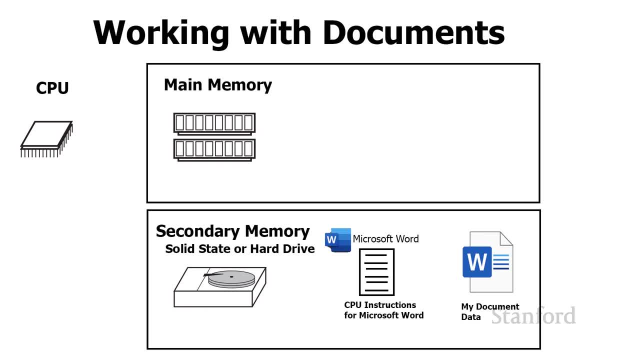 So that needs to be on the secondary memory device. Now, when I actually start editing that paper again, the CPU cannot access things directly from the secondary memory device. So all the contents of my paper need to get copied into main memory When I'm interacting with it, when I'm manipulating it. 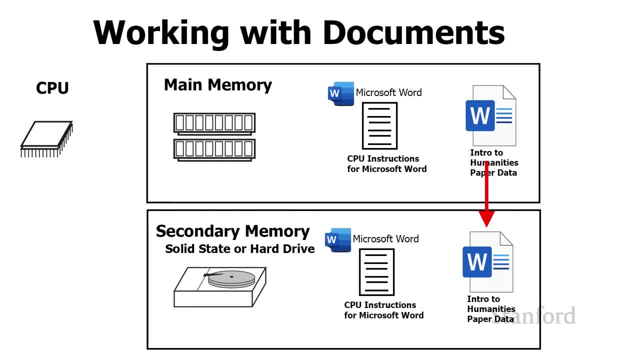 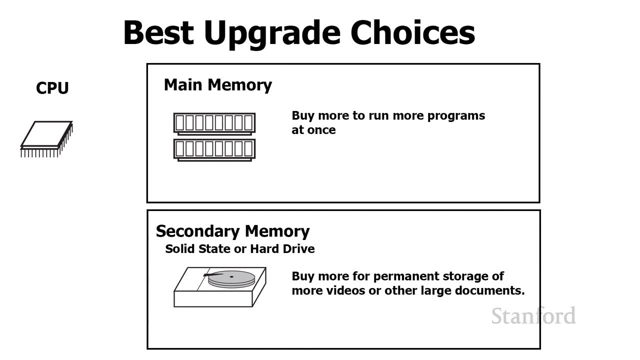 it's in main memory. When I go ahead and save it, it copies everything from main memory. It copies it into secondary storage. So we do need to understand this distinction between the main memory and the secondary storage. Now one question that comes up is: how do I know? 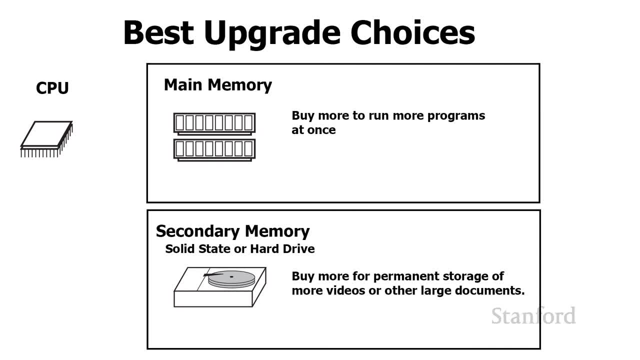 My computer's not acting as quickly as I'd like. What should I do about it? Do I need more main memory or do I need more secondary storage? Well, In general, you're going to need more secondary storage if you're storing a lot of data. 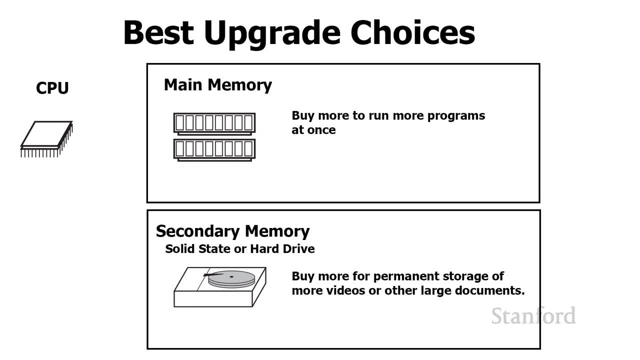 So let's say, for example, you decide you want to be a vlogger, So you're going to do I guess they're called vloggers. Let's just say you decide you want to become a vlogger, You're going to have a whole bunch of video. 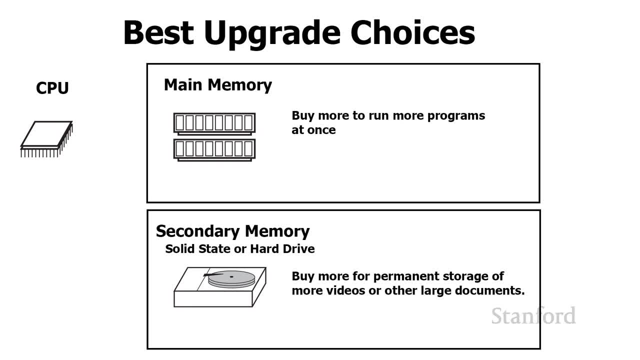 That video is going to take up a lot of space Now. it's not like you're going to have all that video playing at the same time. If you're playing all that video at the same time, then it all needs to be in main memory.